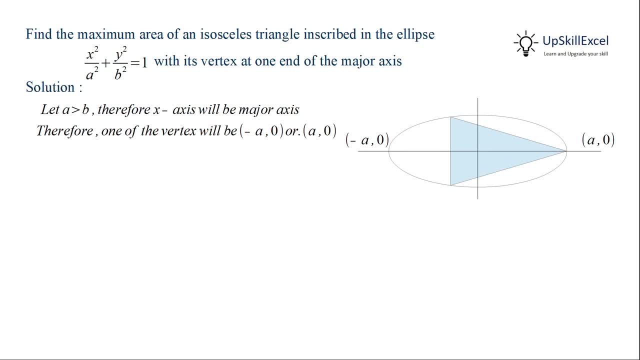 to lie on the major axis. The two vertex can be minus a comma 0 or a comma 0.. Let's take a comma 0 as the vertex Now. as the triangle is an isosceles triangle, the other two vertices will be: 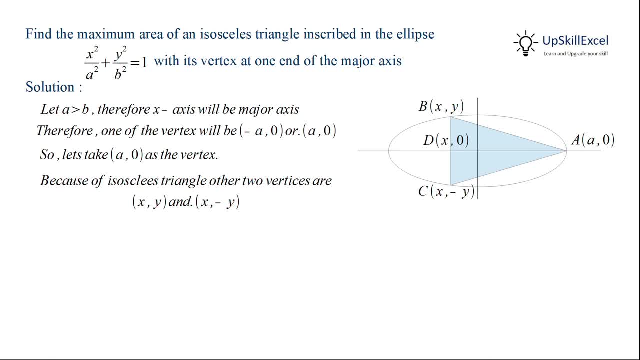 b and c. So let the coordinate of b be x comma y and by symmetricity the coordinates of c will be x comma minus y. Now let's observe the equation of the ellipse From this. by rearranging we will find out y in terms of x. So we take x square by a square to the right hand side, then multiply both. 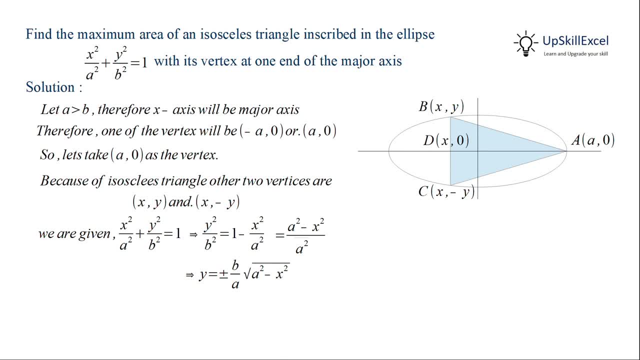 the sides with b square and then, after taking a square, we will get a square. So we take a square and then, after taking a square, we will get a square. So we take a square by a square and then, after taking a square root, we get y is equal to plus minus b by a under root of a square, minus x square. 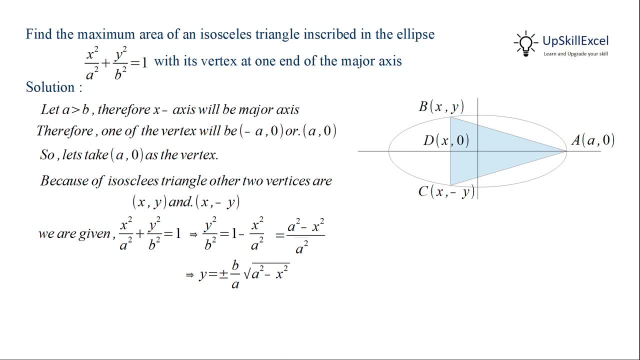 where the positive y corresponds to vertices b and negative value corresponds to the vertices c. Now the base of the triangle is bc, So the length of the base will be equal to the distance between the two points, which is equal to 2y, and the height is equal to the distance between point a and point. 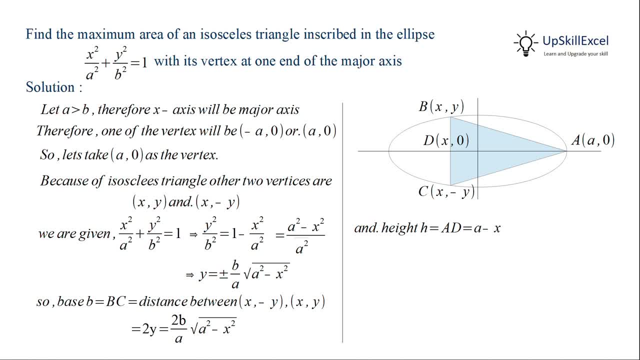 d. Now we have got the height and base, So we can find out the area of the triangle, which is equal to half of base, into height. Substituting the values of base and height and then cancelling out the two, we get area is equal to b by a under root of a square minus x, square multiplied by a minus x in. 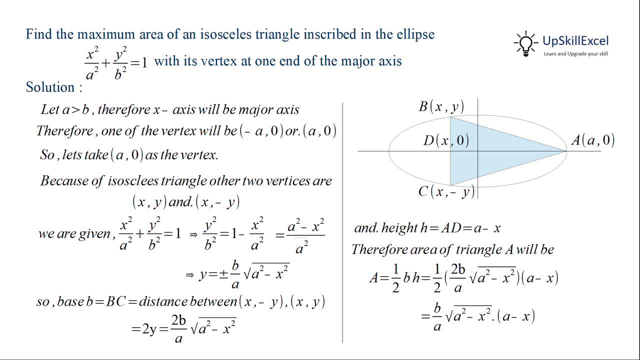 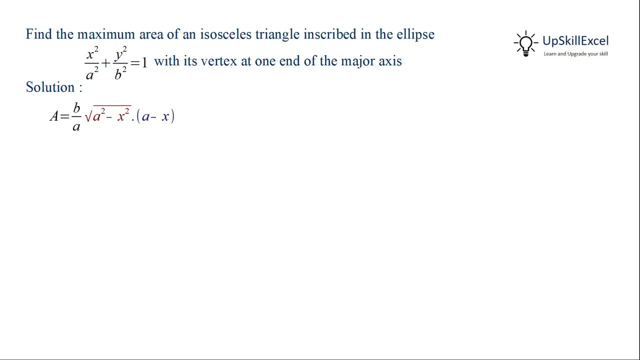 bracket. Now to maximize the area, we will differentiate area with respect to x. Here, on the right hand side, we have two points which are equal to b by a under root of a square minus x square multiplied by a minus x in product. So we will apply product rule differentiation. Now we know that derivative of under root of a square 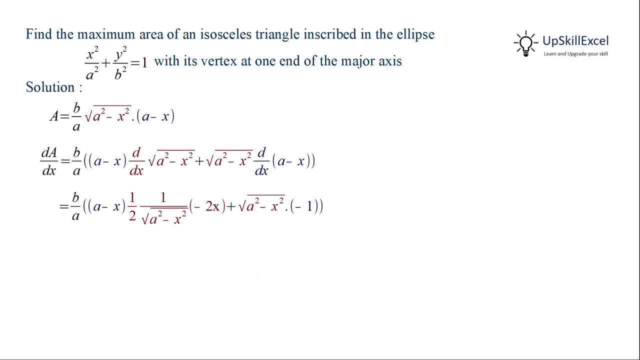 minus x square is half of 1 over under root of a square. minus x square multiplied by minus 2x. The minus 2x comes from the chain rule by differentiating minus x square. Similarly, derivative of a minus x is equal to minus 1.. Now we can simplify this by taking the common denominator under root of a.